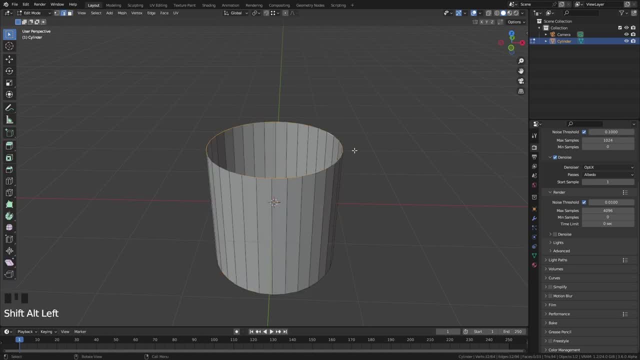 just delete the top of a cylinder and then you select the top edge loop, You press E to extrude and S to scale it in a little bit, And then, if you press CTRL-F with the inner ring selected, you can perform a grid fill operation. 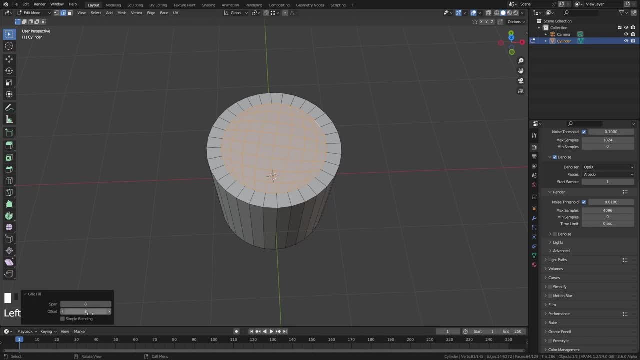 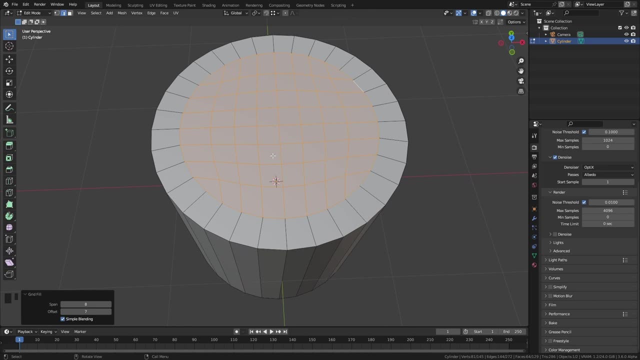 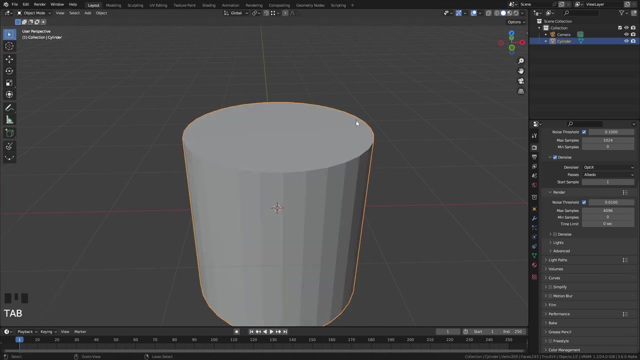 You can straighten this out a little bit, if it's wonky, by playing with the offset number, and I tend to find that you get slightly better distribution of faces if you enable simple blending In object mode. if I press CTRL and a number like 4, that'll add a subdivision surface. 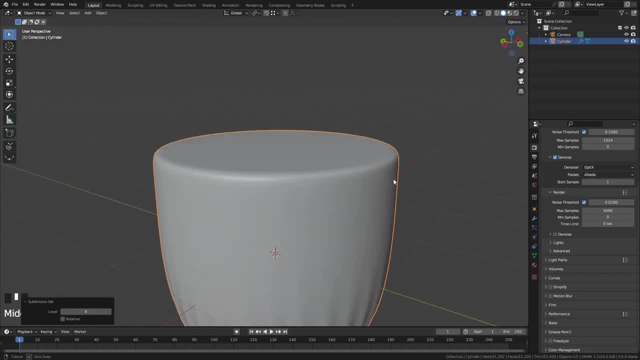 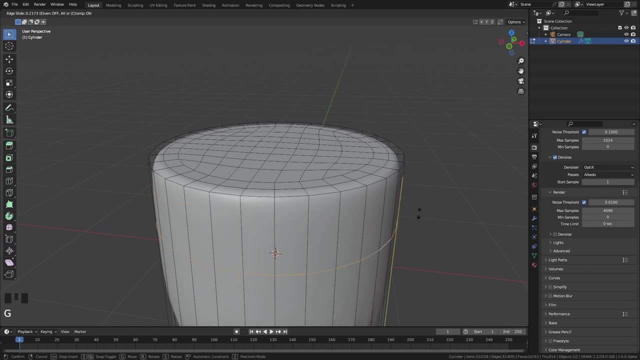 modifier and I can add some support loops and, as you can see, we get some nice shading and good quad topology. We can also easily change how sharp the edge of the cylinder is just by grabbing these edge loops and double tapping G and then sliding them closer or further away from the 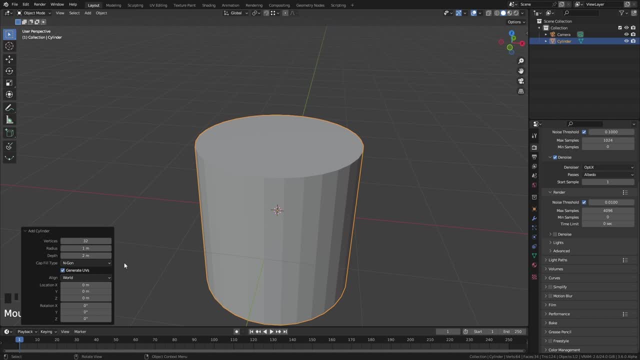 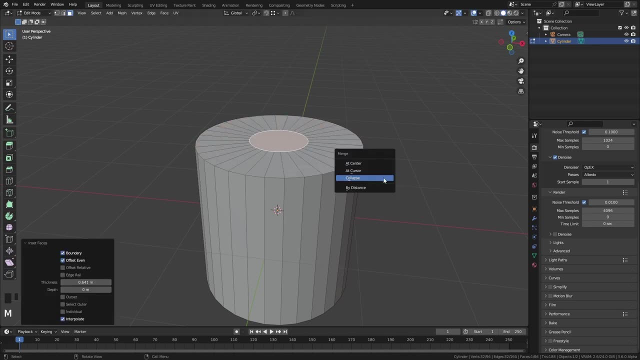 edge. The next method requires you to have a cylinder that has a triangle fan. There is an option for that when you make the cylinder, or if you've already got the cylinder in the scene, you can select the top inset a little bit, press M and collapse, and you'll get a triangle. 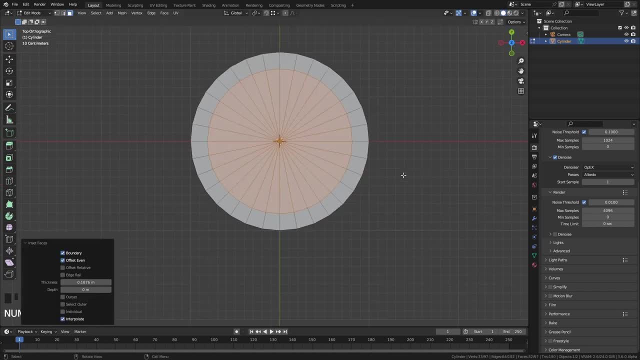 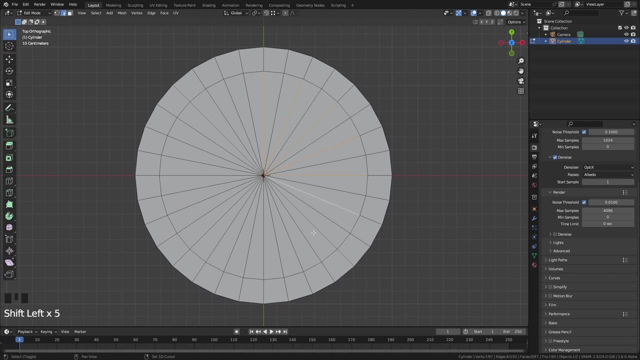 fan. So if we select the top and we inset again, then we just need to go around and manually select every other one of these edges that make up the triangles. Unfortunately, check a decent number of times. I've used the same method a couple of times, but I've 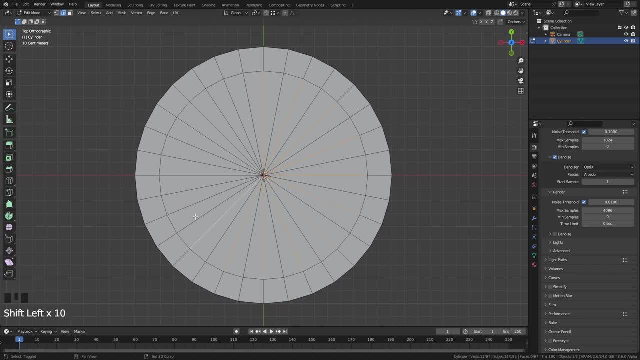 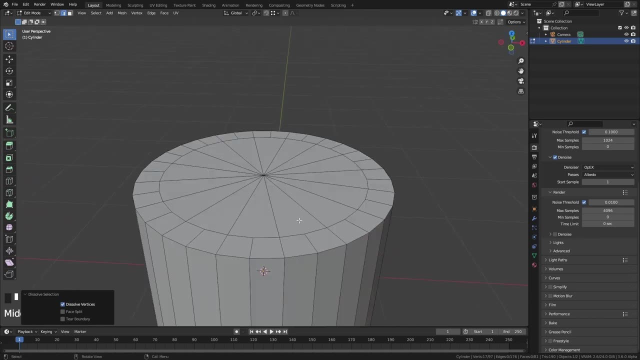 had to check a de-select and things like that won't work here, so you do have to do it manually, but it doesn't take very long. Once you've got that done, you can press CTRL and delete, which will dissolve those edges. 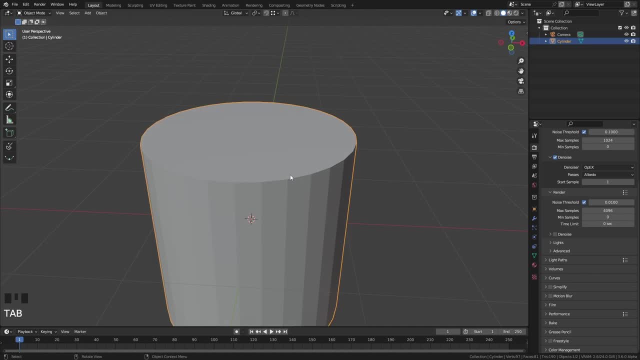 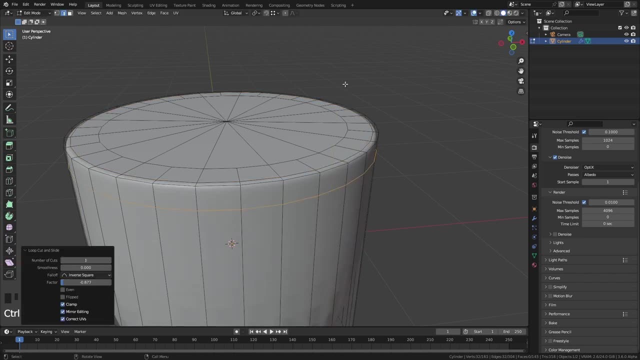 and now the triangles are actually all quads. So we can add in a support loop to this. because if you look, if we add the subdivision surface, you can see it goes a bit wobbly. but if we add support loops in we get a nice smooth top on the cylinder. 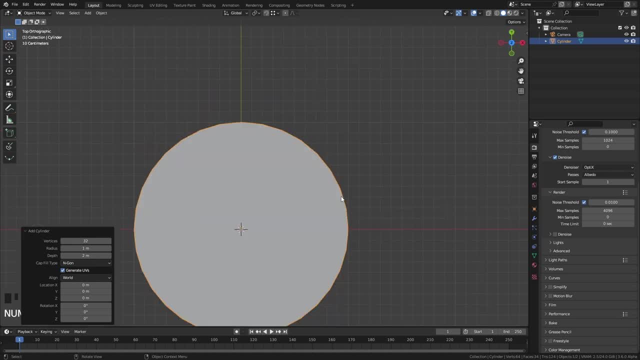 So for this final method, we're just going to need a little bit of a bit of a workaround. We're going to need a little bit of a workaround. So for this final method, we're just going to need a plain cylinder. I'm going to go into top view with number pad seven. I'm going. 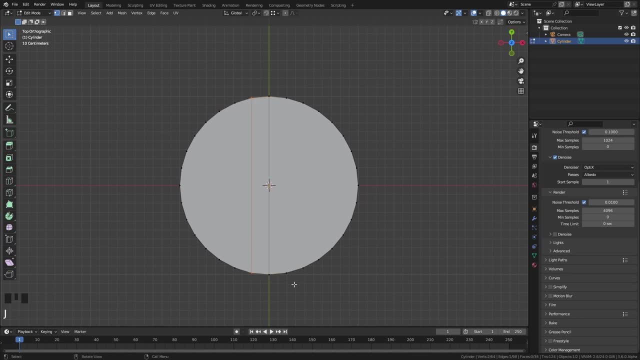 to select the top and bottom most vert and I'm going to press J to join them. Then we're going to do that one vertex either side. I'm going to do 11 horizontal cuts, So I'm starting with the middle row and I'm doing five above and then I'm going to go down and select the. 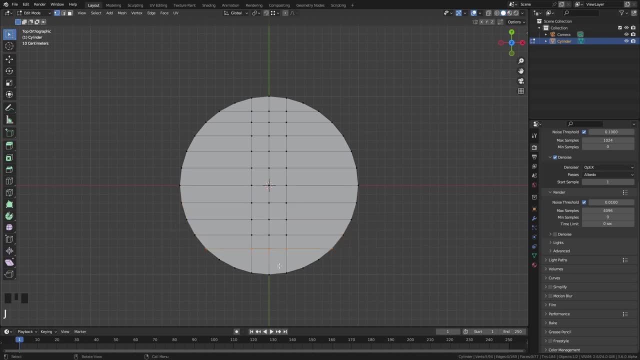 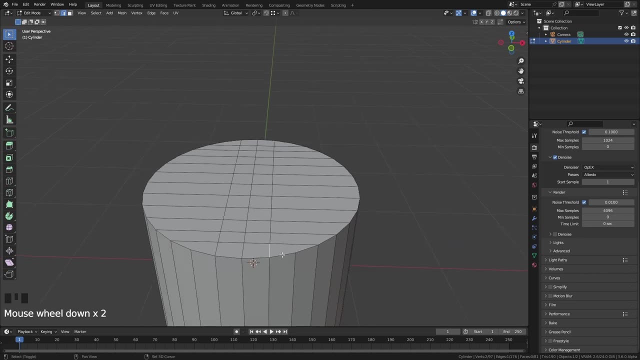 ones underneath, and I'm going to do the five below. If you don't connect the last one together, then what you'll notice is that that face is actually a quad with four sides on the edges. So now, like before, we can just add in our supporting loop. We can select all of the 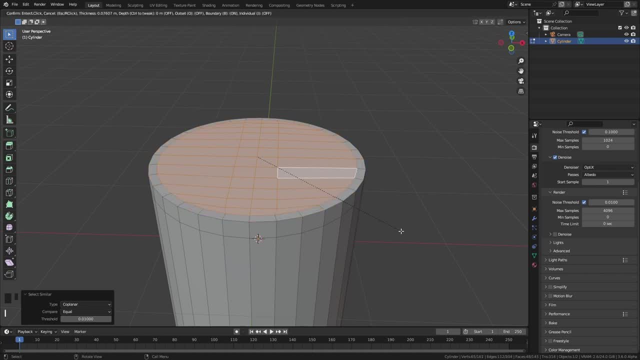 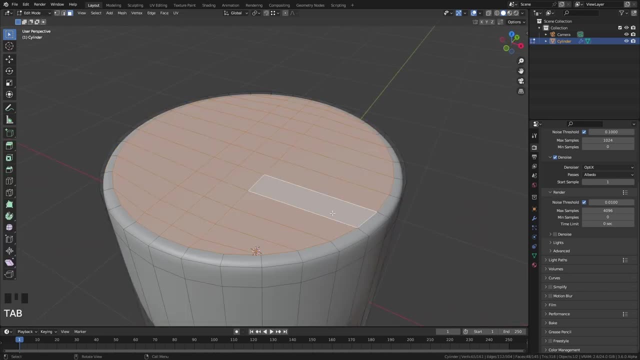 faces on the top and do an inset with the I key to add a supporting loop around the top as well, And if we add a subdivision surface modifier, we get another nice, smooth result. Now I don't use this one very often, but it can be handy when you need to transition from. 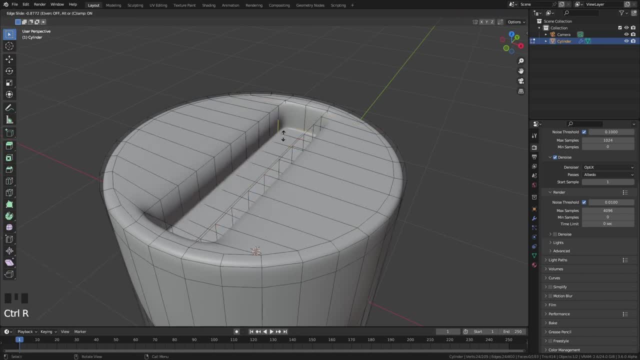 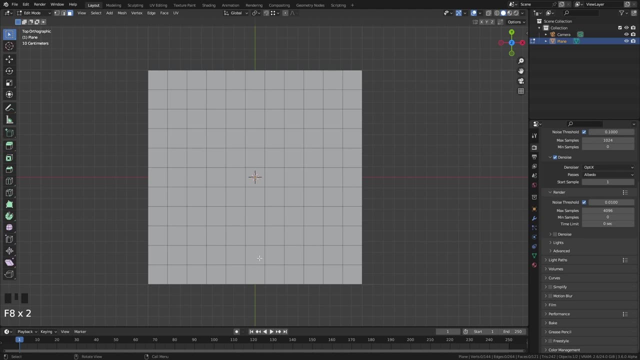 a cylinder to a square shape. Subdivision surface modifier. like this you can make these nice inset shapes, which sometimes comes in handy. OK, so this mesh has edge loops that go horizontal and it has vertical ones, But what if we wanted to change the direction of a loop so it goes something like this, around a corner? Well, 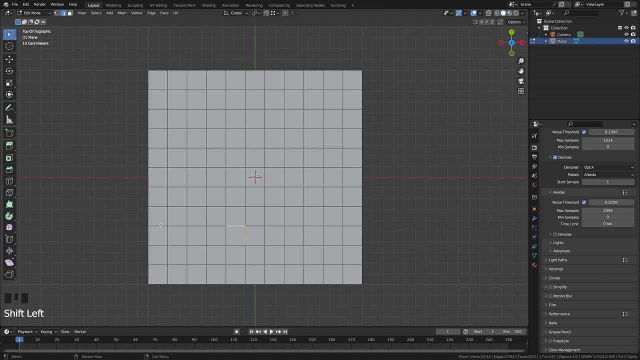 that's actually quite easy to do. All we need to do is select the two edges that we want to become our redirection point, press M and collapse. In theory, we have just done exactly what we set out to achieve. We've redirected a loop to go around a corner. You can see. 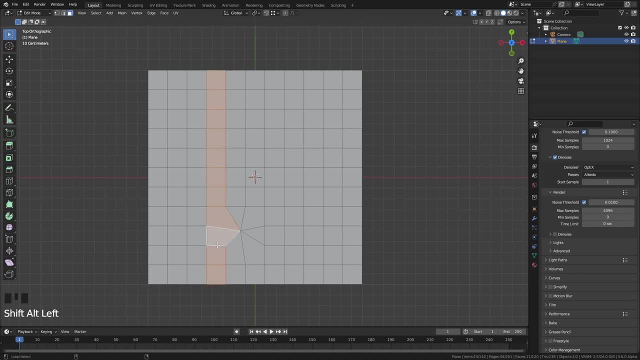 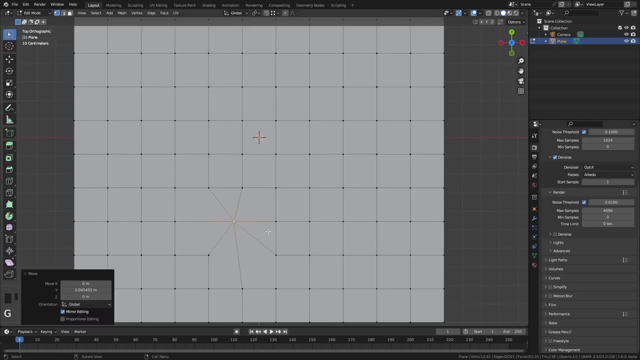 that we still have edge loops that go horizontal and we have vertical ones, but we now have an edge loop which turns the corner. However, this looks really bad and it's messy topology, So I'm just going to use the snapping tools to align this with the other verts around. 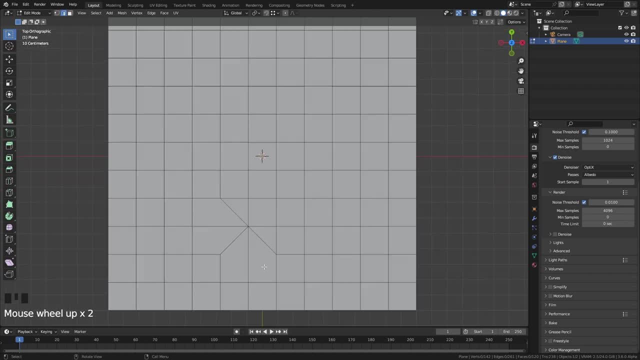 it to move it into a bit of a better position. You can see that we've created two triangles here as well. All I'm going to do here is just select these two edge loops and press control and delete And just dissolve them entirely. Now we have the really nice, clean topology that we were 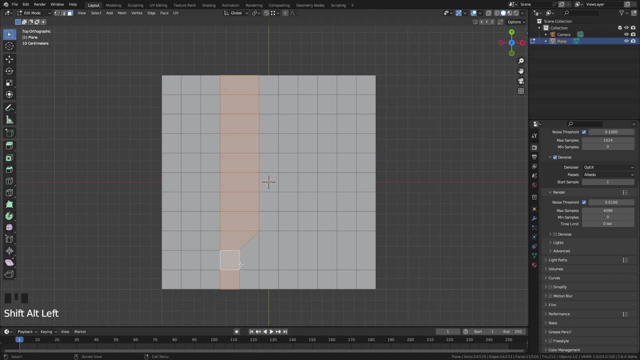 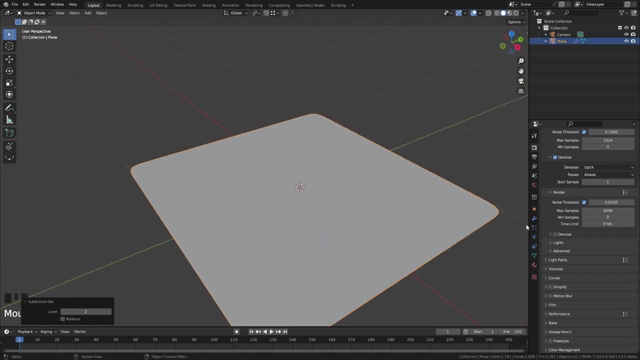 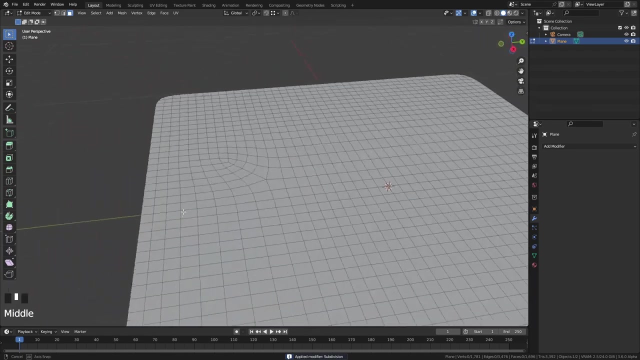 looking for and we still have that redirected edge loop with one going horizontal, one vertical and one around the corner. If we apply a subdivision surface modifier to this, you can see that we get some pretty decent looking topology and it's a nice smooth curve. 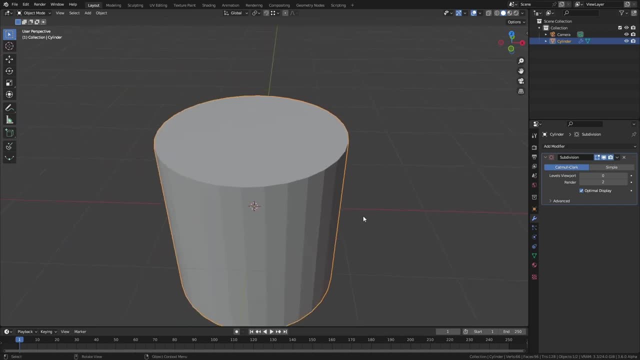 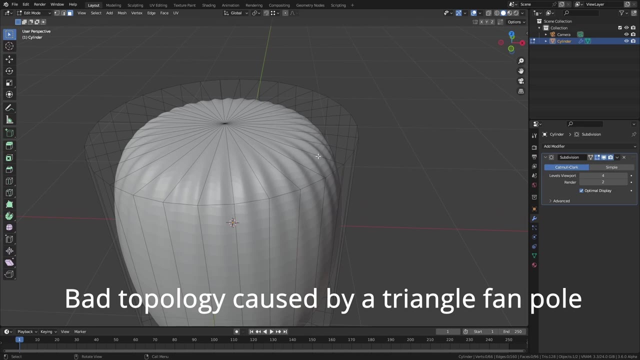 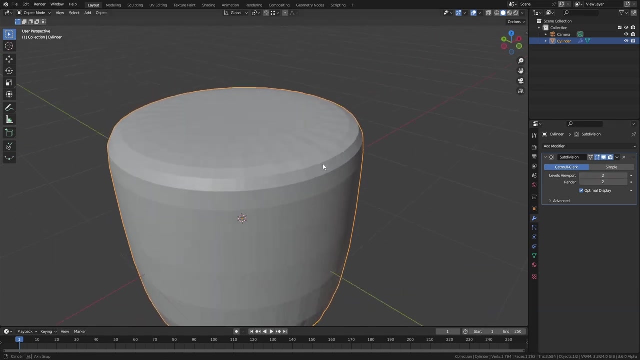 The next thing I want to talk about is dealing with poles. A pole is a vertex connected to multiple edges. As we've learned about in 3D modelling, there's N-poles, which have three edges, and E-poles, which are connected to five edges. Poles with six or more connecting edges are usually considered. 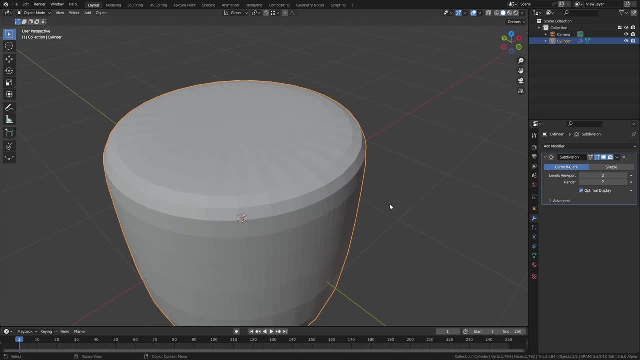 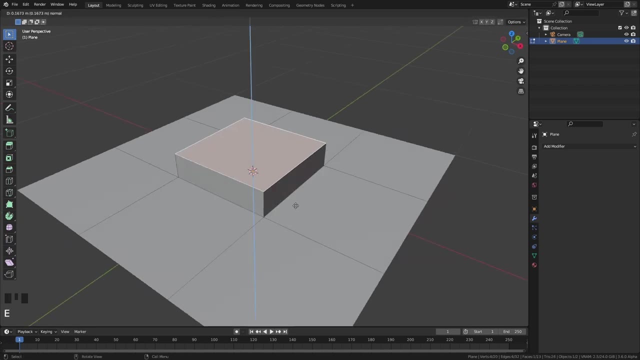 bad topology and should just be avoided entirely where possible. E-poles, the ones which have five edges, are most commonly created when you extrude a face out, and N-poles, the ones with three edges, are most often found on sharp corners. Now, poles aren't necessarily. 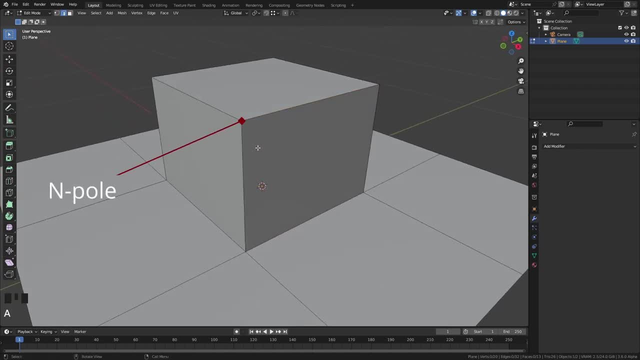 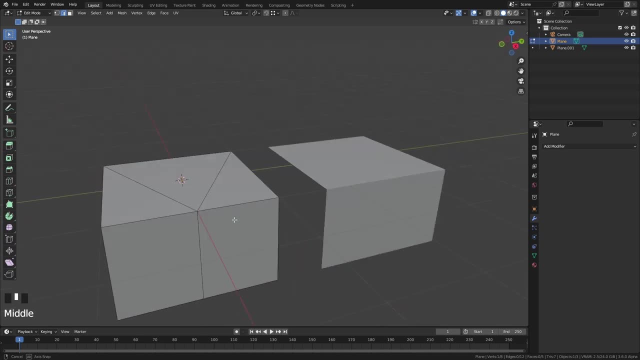 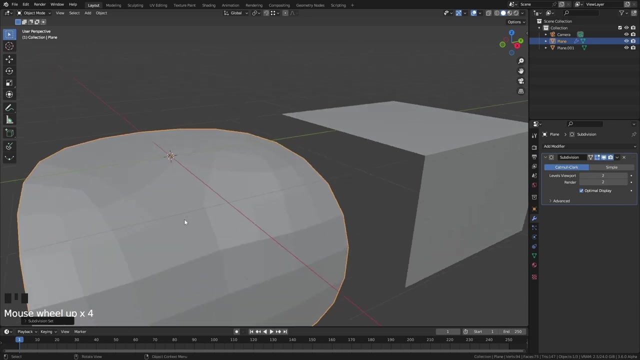 bad. They're actually unavoidable. However, you do need to manage them properly to make sure that they don't cause shading issues and other mesh artefacts. Generally speaking, you should avoid placing either type of pole on a curve with a steep gradient. Try to move the pole away to a flatter area of the mesh instead, For example here: 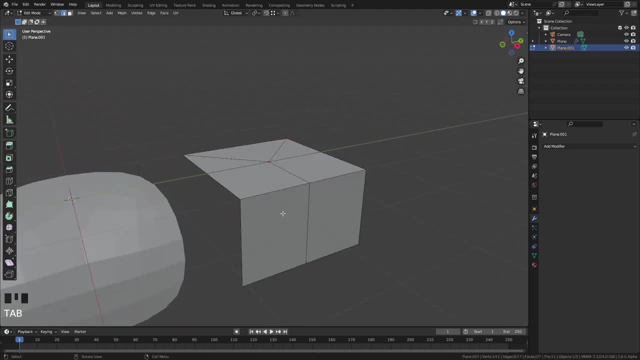 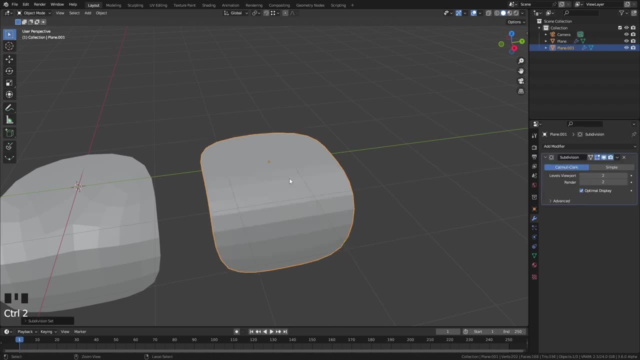 is a mesh with an E-pole right on the corner and you can see, once we apply the subdivision surface modifier, it causes this weird pinching effect. Now here's the same mesh, only I've moved the pole so that it's further back from the curve and now on a flat surface. 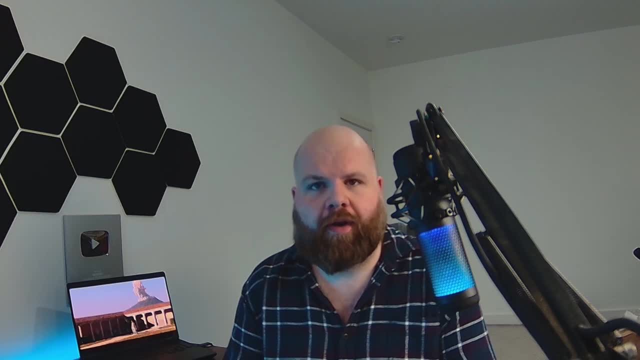 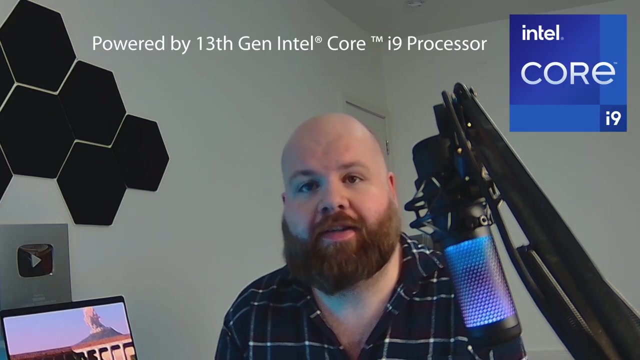 which completely eliminates all the problems. Before we move on, I want to take a minute to talk about the sponsors of this video, Asus and Intel. They've sent me this. It's an Asus ProArt StudioBook 16 OLED laptop. This thing is a real beast for creative work. It comes with a powerful Intel Core i9-13980HX. 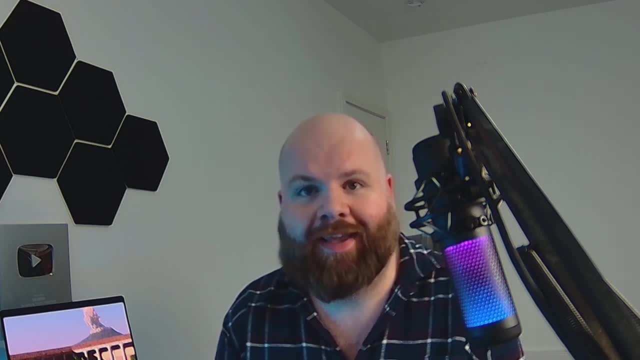 processor, An RTX 4070 graphics card, 8TB of storage. It comes with a powerful Intel Core i9-13980HX processor, An RTX 4070 graphics card, 8TB of storage and 64GB of RAM. 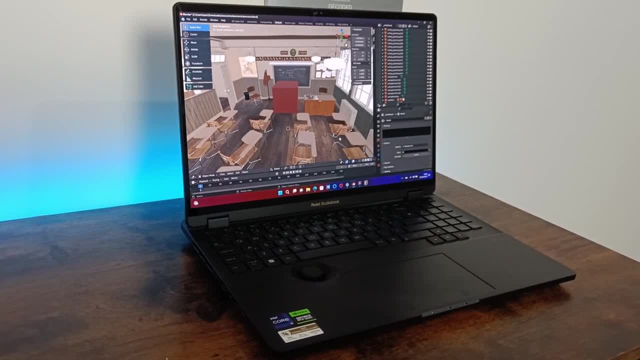 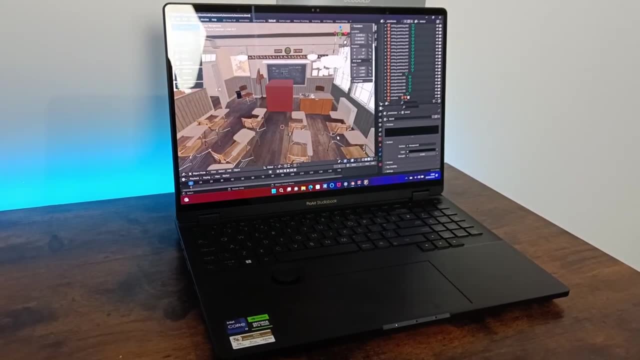 It's powered by a 13th Gen Intel Core i9 processor, and the 16-inch Asus Lumina OLED display looks absolutely gorgeous. It's 3.2K resolution, touch compatible, and the laptop comes with a stylus in the box, which is really handy for 3D work. 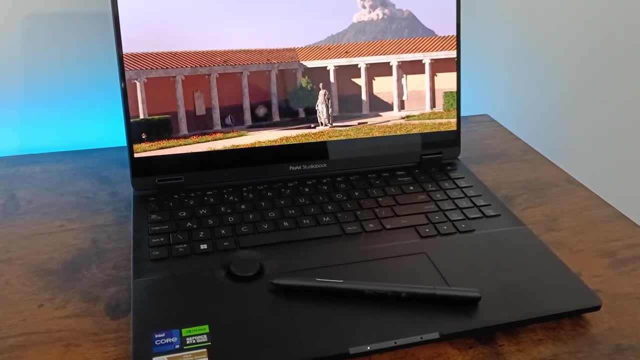 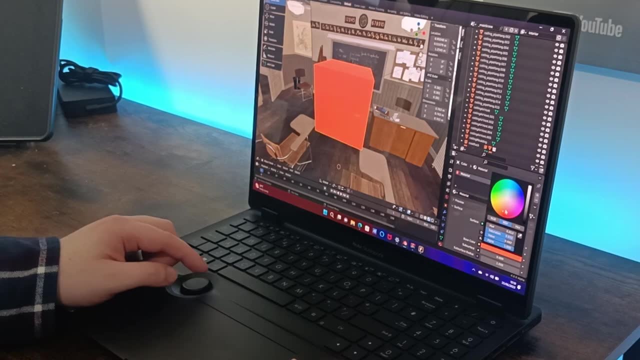 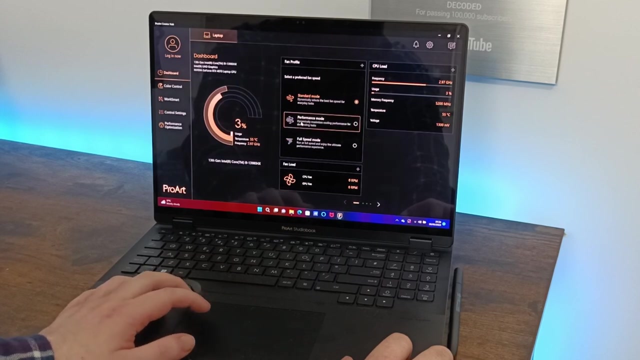 Another great feature, specifically for 3D artists, is the inclusion of a dial for precision control when adjusting parameters like colours and brush sizes. The Asus dial has a lot of useful applications that can be adjusted in the Asus ProArt Creator Hub app. This is an application that makes it really easy to calibrate and customise. 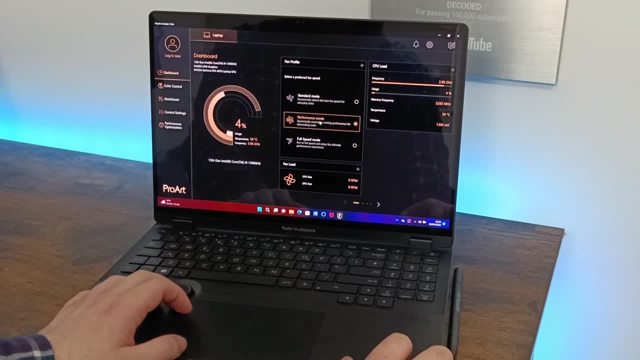 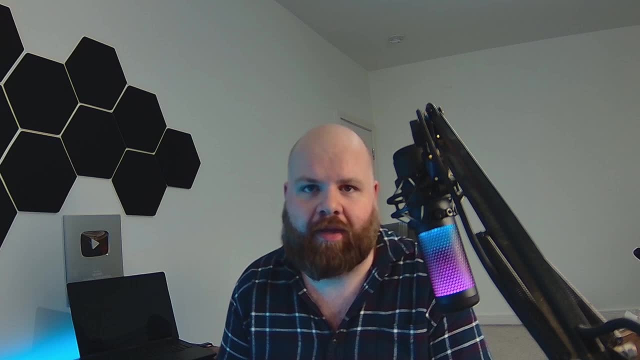 your device as well as monitoring its performance. I'll be spending the next few weeks putting this laptop through its paces with a really ambitious project, so keep an eye out for that video. You'll find a link in the description where you can find out more about this Asus laptop and the Intel processor that powers. 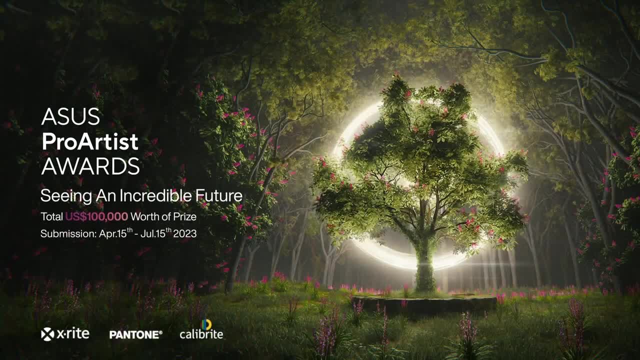 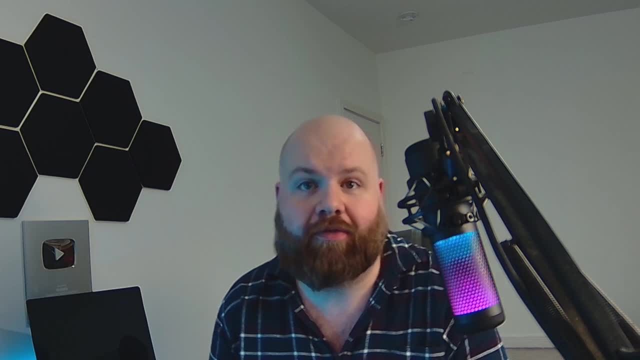 it. If you want to check out the Asus ProArtist Awards for 2023, it's currently open for submissions. It's always a fantastic competition and the total prizes this year are worth more than $100,000.. Topology of the human face is one of the more daunting exercises in 3D modelling. It's 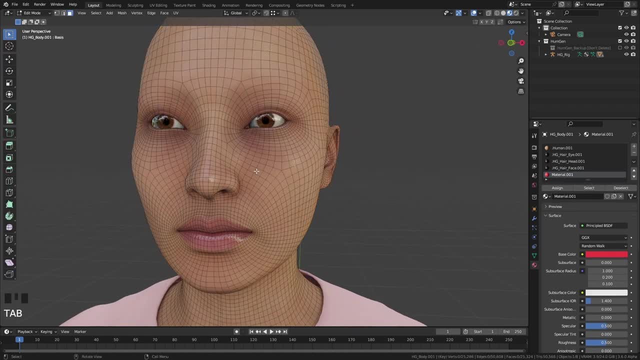 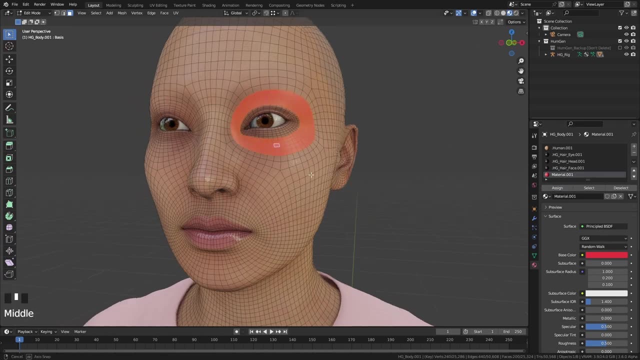 a very complex shape to begin with and you need to think about how the mesh will deform when it's animated and you also want to avoid any weird shading artefacts. Over the years, 3D modellers have devised a fairly standardised method of face topology. 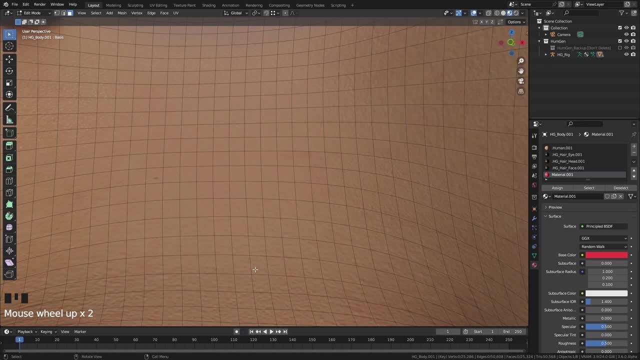 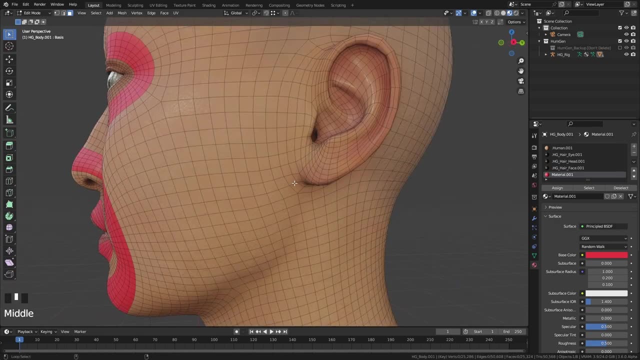 So one edge loop should go around the eyes. another loop goes around the mouth, A wider loop goes around the chin and across the bridge of the nose, and then there's a fourth loop that usually surrounds the ears. Then it's just a case of expanding these loops and joining. 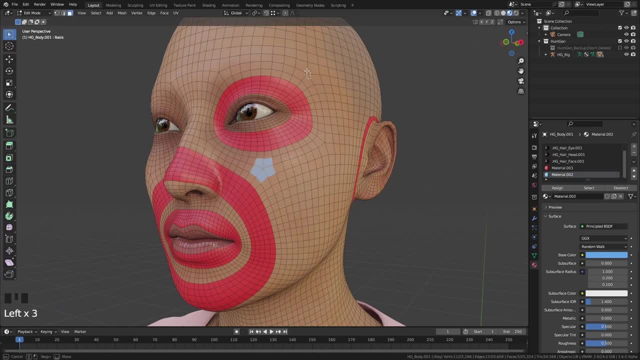 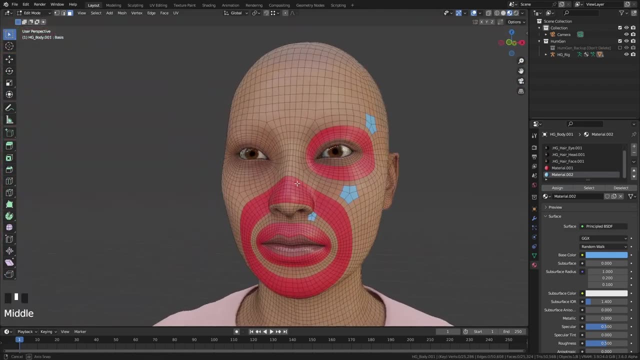 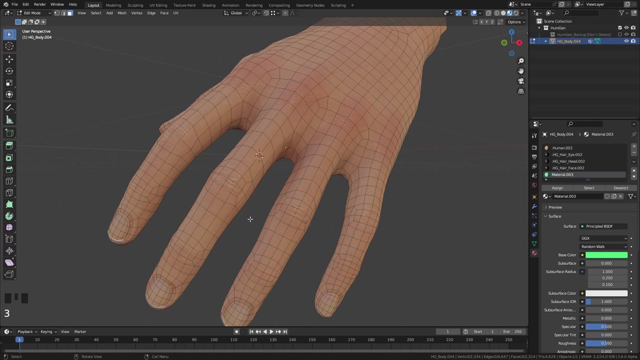 them together. You'll notice where the loops do join. it creates epauls. This method puts the epaul in the least problematic areas. They're inevitable, but if you use this loop arrangement it shouldn't cause any issues. b- This final tip is a really quick one. When you're making a deformable joint on a character. 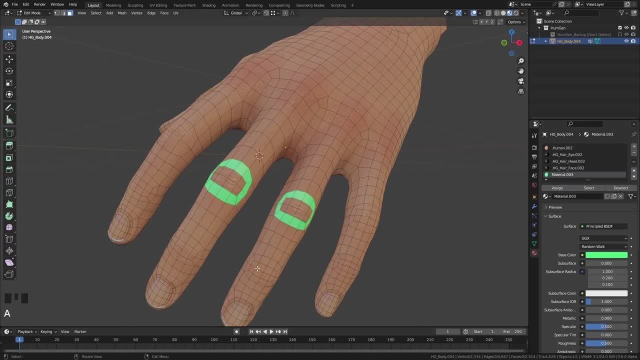 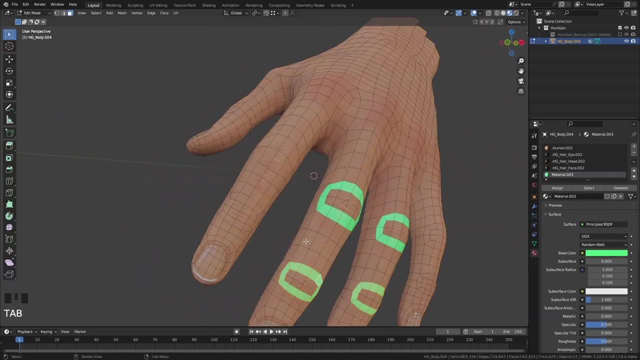 such as an elbow, a knee or a finger knuckle, it's important to have an edge loop which runs around the circumference of the top of the joint. You can see that here on this human generator model. It's actually very easy to do. you just need to select the top eight.